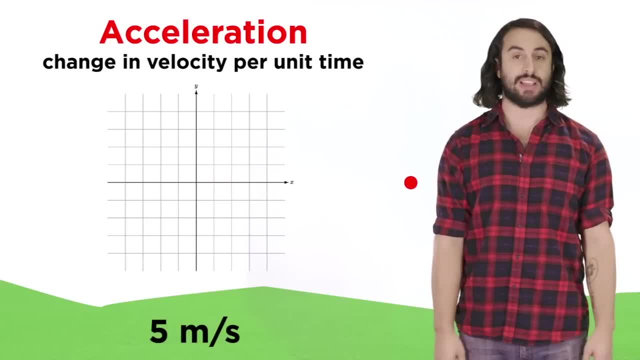 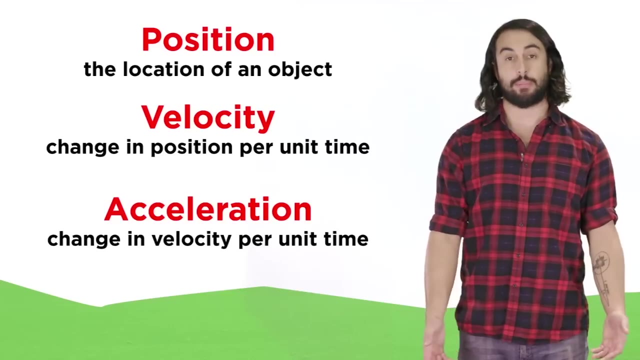 and over five seconds, gradually speeds up to five meters per second. then it is accelerating at one meter per second, per second, or one meter per second squared. So that's how we define position, velocity and acceleration. Now let's discuss each of these in more depth. 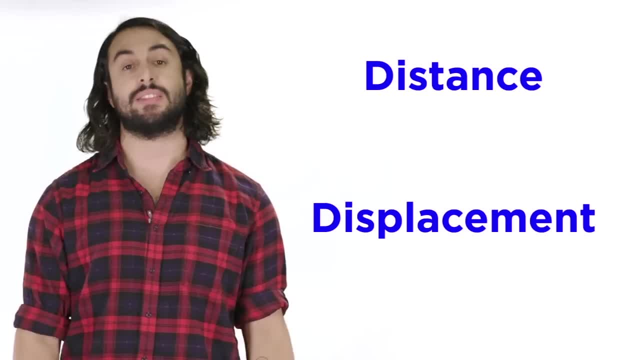 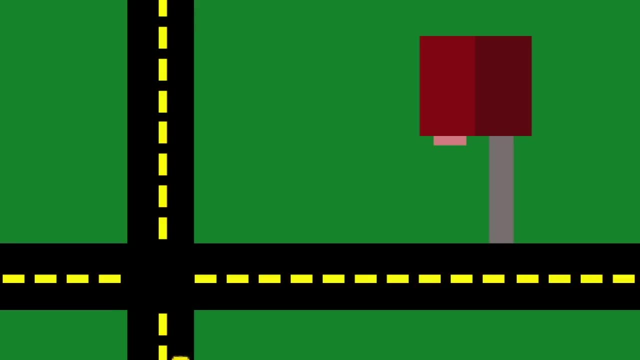 When we talk about position, we could discuss distance or we could discuss displacement. The difference here is that distance is a scalar, while displacement is a vector. Let's say, you and your friend get dropped off by the school bus at this intersection. 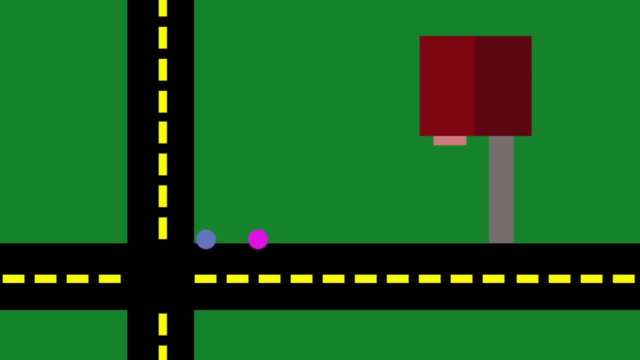 and your house is here. Your friend begins to walk down the street and up the driveway like a normal person, But you find yourself so overcome with excitement to play video games that you decide to plow through the yard in a straight line, A straight line to the door. 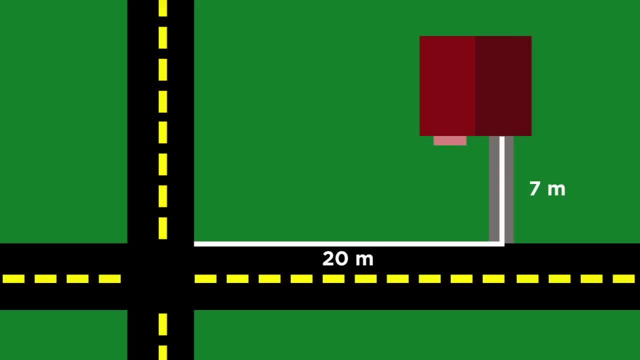 Your friend has to walk twenty meters down the street and seven meters up the driveway, for a total of twenty-seven meters. So using the Pythagorean theorem, we find that you only had to walk about twenty-one point two meters, and you probably got there a little sooner. 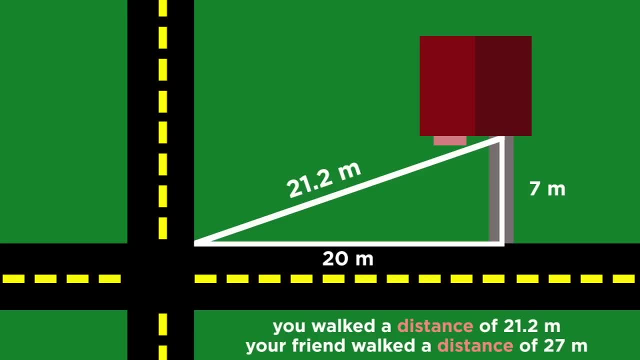 What we can say is that you walked different distances, which are represented by these scalar values, But you both had the same displacement. That's right Displacement, because you ended up in the same spot, at the front door. This vector, which follows the straight line path, is the displacement vector for both. 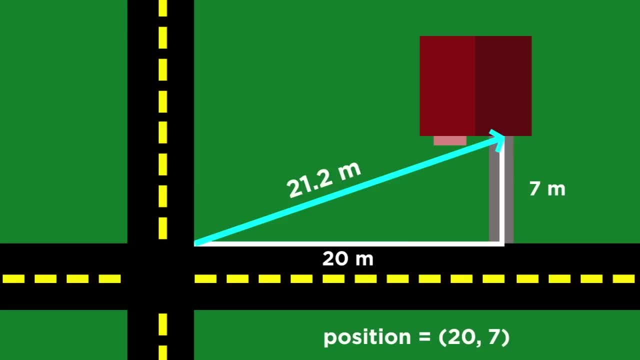 of you and we can report your position with X and Y coordinates like this: twenty comma seven. Or we could report the magnitude of the displacement vector, which will be equal to the shorter distance you traveled, and calculate the angle off the horizontal using trig functions. if 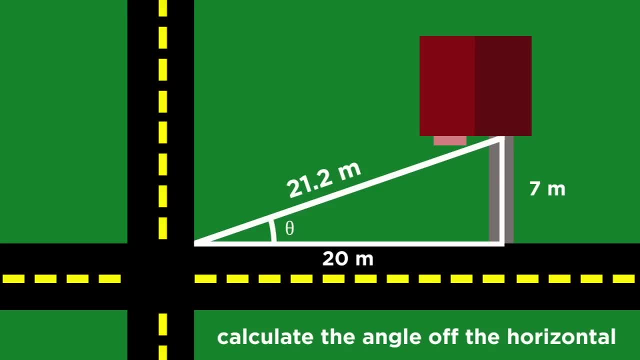 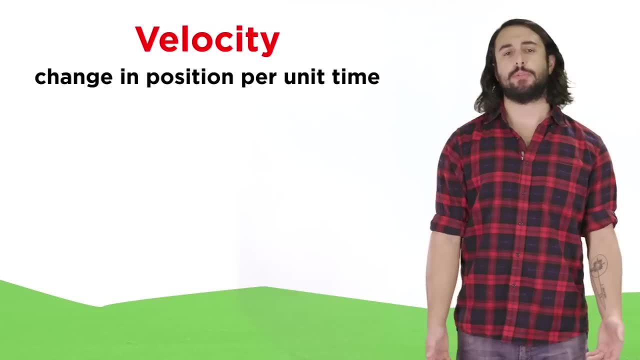 we desire In order to report the direction of the vector. Next, let's look at velocity, which is the rate of change in position. Most people assume that the words speed and velocity are synonyms, and in everyday language they are, but the difference in physics is that speed is a scalar and velocity is a. 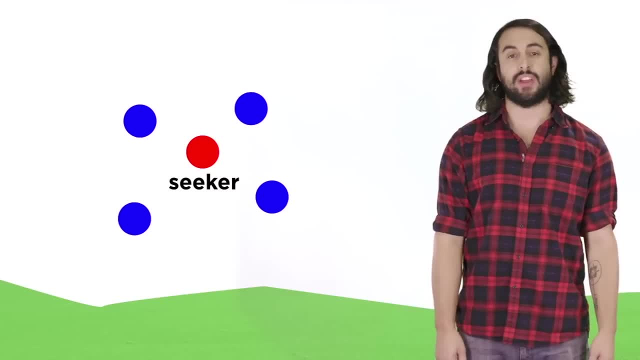 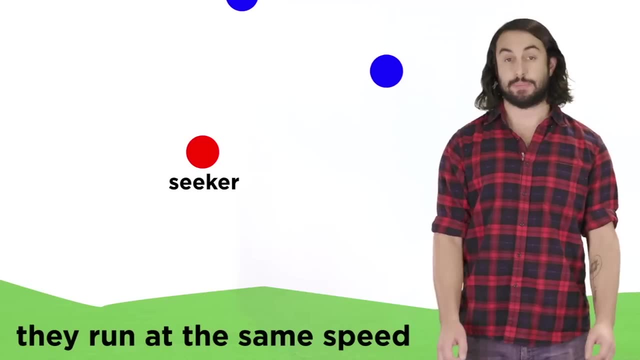 vector. If a group of kids are playing hide and seek and they all run away from the seeker in different directions, it is possible that they all run at the same speed. So the speed is the vector. Speed is the vector. Speed is the vector. 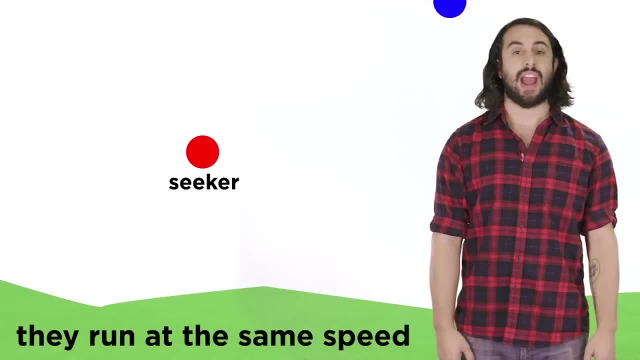 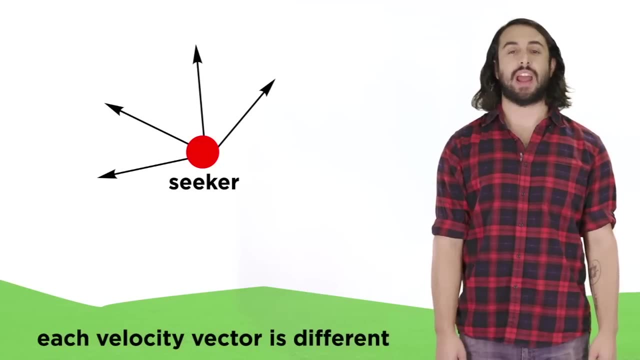 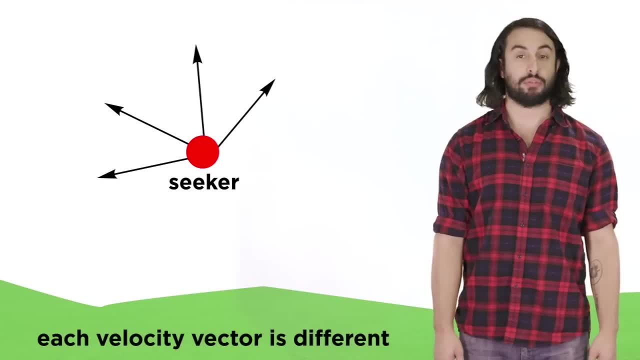 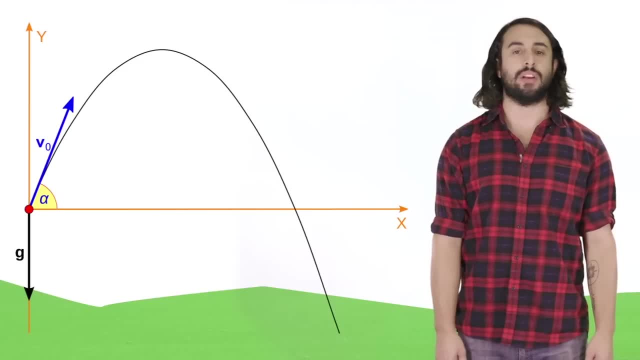 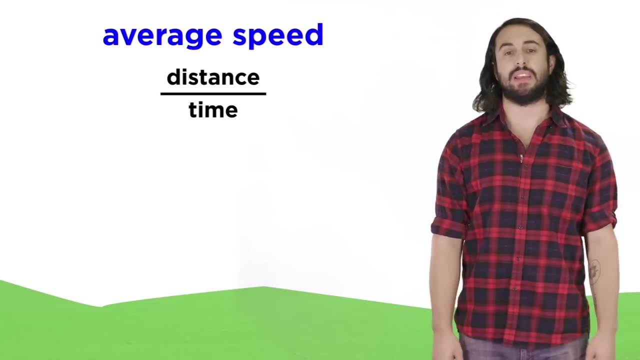 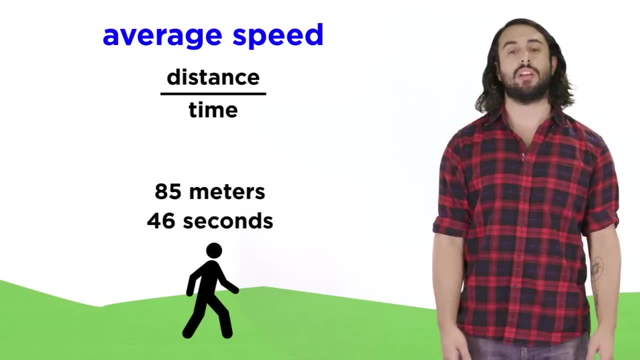 and dividing by the time it took to do so. So if you walk 85 meters in 46 seconds, you are walking at an average speed of 1.85 meters per second. To find average velocity, you can do the same, but you would have to divide displacement. 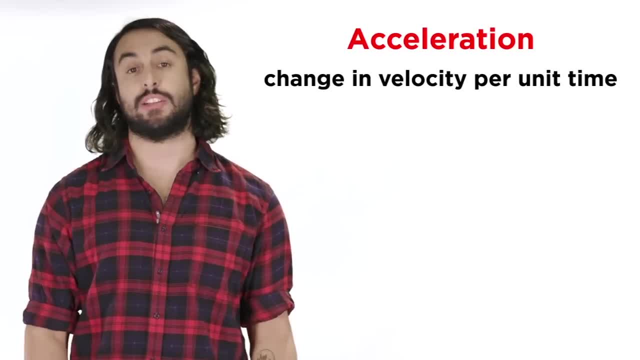 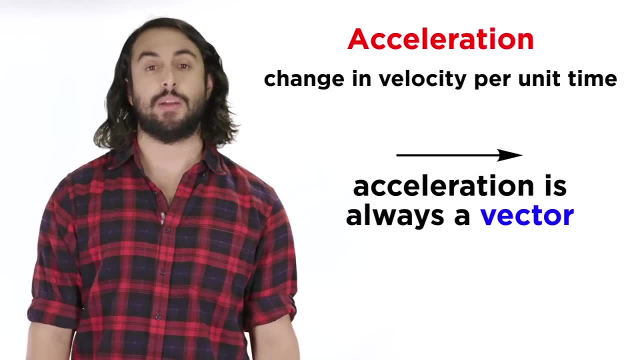 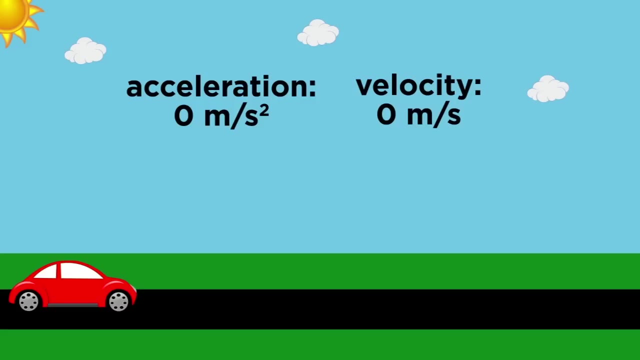 by time. Lastly, we have acceleration, which is the rate of change in velocity. This is always a vector, because acceleration must occur in a particular direction. If you are in a car that is standing still and you press on the gas, the car will begin. 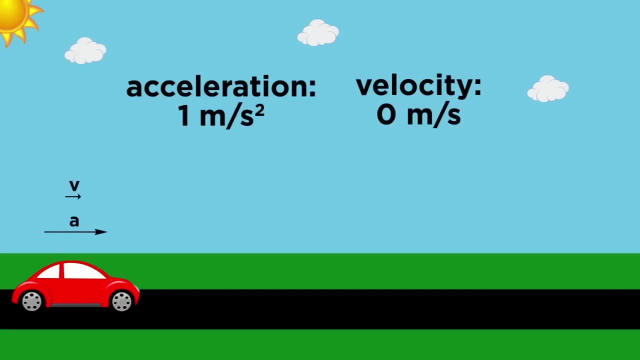 to move forward with a fixed acceleration. It might accelerate slowly, so the vector may be on the shorter side, but this constant acceleration will cause the velocity to increase at a fixed rate. Let's say an additional meter per second every second, so over 5 seconds it will reach. 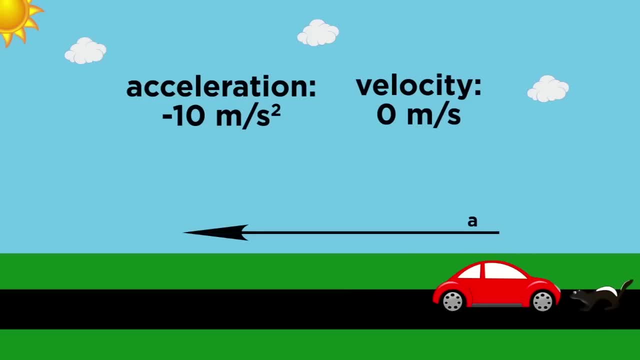 a velocity of 5 meters per second. Let's say you see a skunk in the middle of the road. It's your most favorite animal, so you slam on the brakes. We can describe this as a deceleration, which is an acceleration in the negative direction. 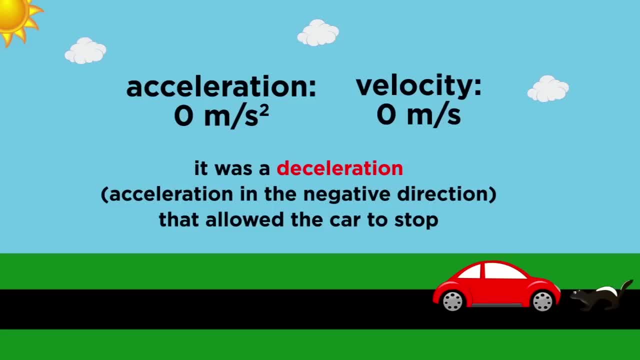 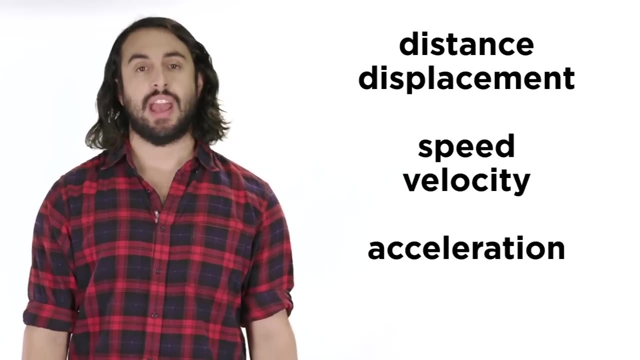 Since you are going from a moderate speed to a standstill in a very short amount of time, this vector will be quite long and pointing back towards the origin. Now we understand distance and displacement, speed and velocity and acceleration, and we can categorize these as being either scalars or vectors.